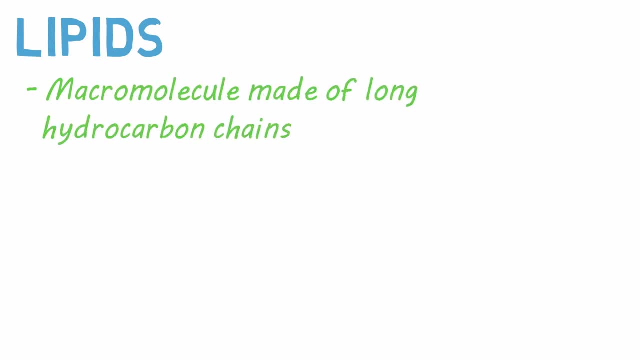 Lipids are macromolecules made up of long hydrocarbon chains, thus named because they are made up exclusively of hydrogen and carbon. These long hydrocarbon chains give lipids their nonpolar property, which means they are not soluble in water. This is why oil separates out from water when mixed. 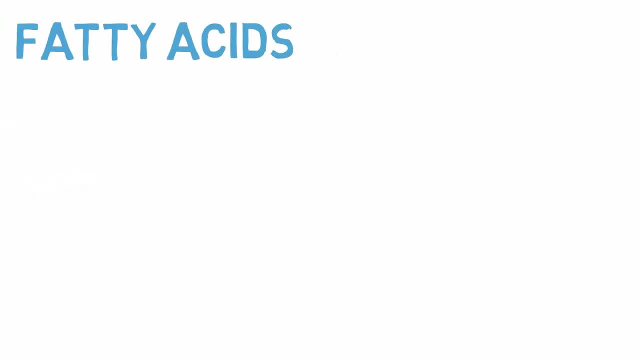 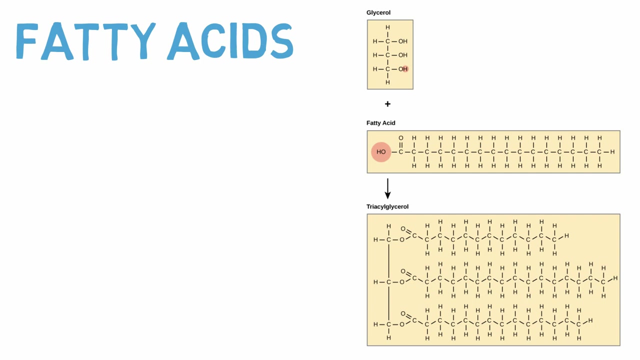 One of the most common components of certain lipids is the fatty acid. Three fatty acids come together with glycerol to form a larger molecule called triglycerol or a triglyceride. Triglycerides have various functions in the body, but a primary one is energy storage as fat or adipose. 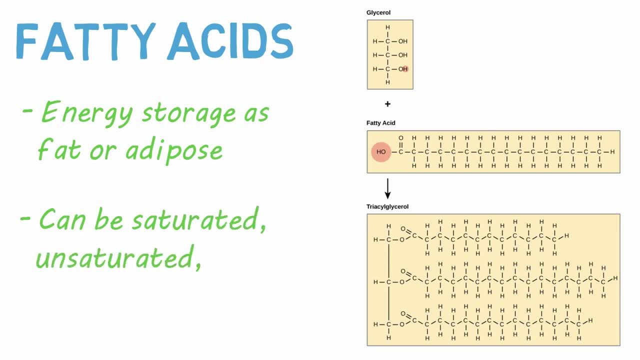 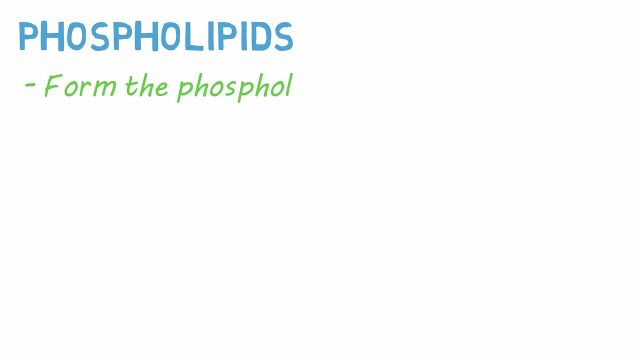 Fatty acids also include saturated and unsaturated fats, trans fats and the omega fatty acids, But they are not the only ones, But we won't go into their detailed differences in this video. Another molecule that incorporates the fatty acid chain is the phospholipid, most famous for its formation of the phospholipid bilayer, which protects a cell from outside intrusion. 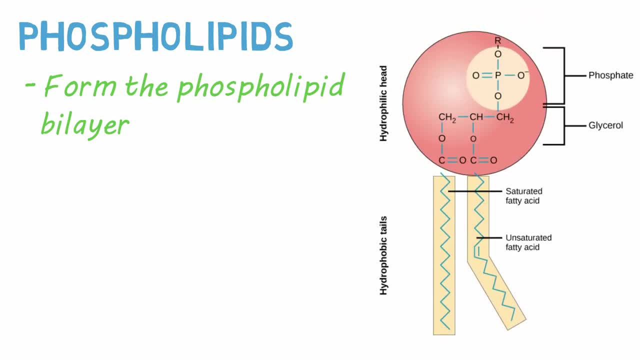 Phospholipids contain two nonpolar fatty acid tails bound to a polar phosphoglycerol head. This is why they form a bilayer, because the nonpolar tails are attracted to each other and the heads are attracted to water solutions in and out. 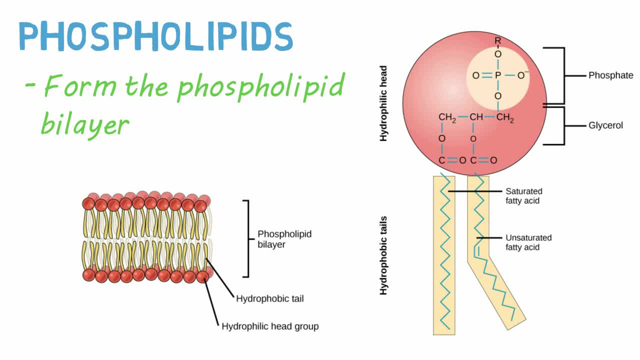 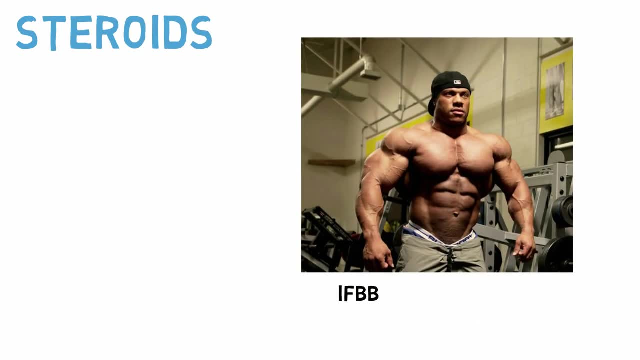 At some point, I'll make a video discussing just how awesome this cell membrane is. Let's talk about steroids next, And yes, this includes these types of steroids, but that's not the focus of this video. Steroids are hydrophobic and not water soluble like other lipids, but they do not contain fatty acids. 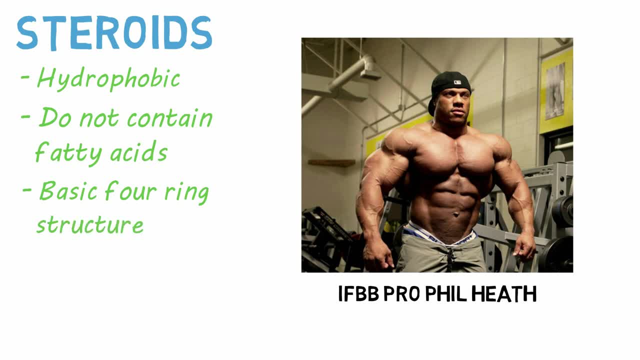 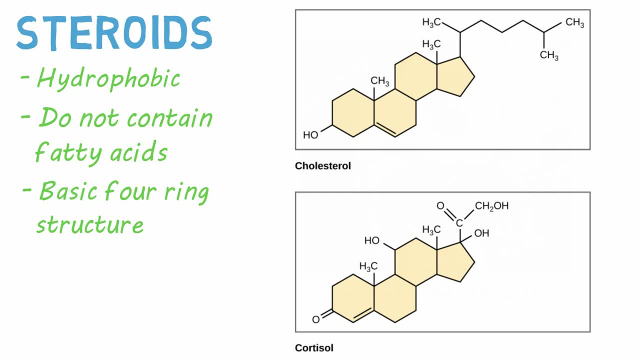 Instead, they have four acyclic rings linked together. This basic structure is then added to to give us common steroids like cholesterol and cortisol. Steroids have many functions throughout the body, including the presence of hormone steroids like progesterone and testosterone, both formed from cholesterol. 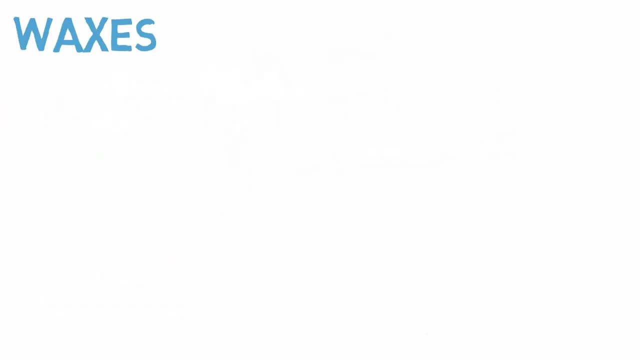 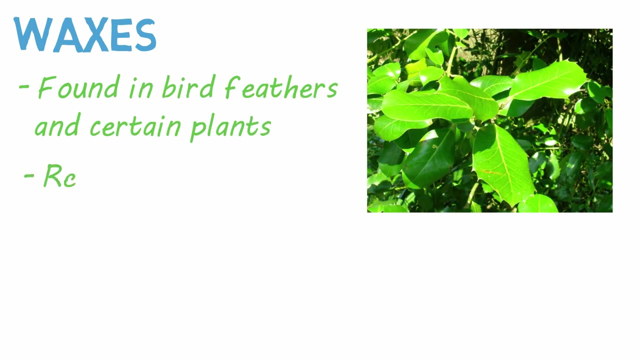 Finally, let's not forget about waxes. Waxes have a variety of unique structures and are found in the feathers of some birds and leaf structures of many plants. This is why water beads up and runs off certain plants. There's a lot more to lipids.